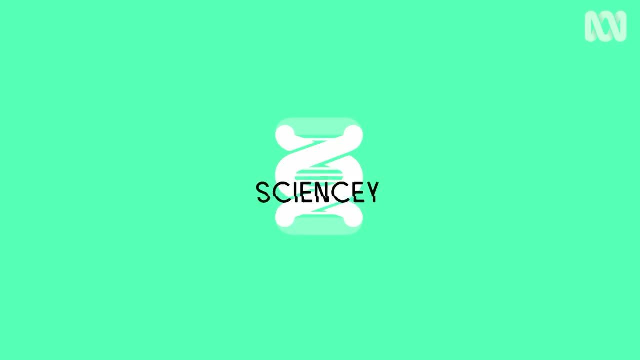 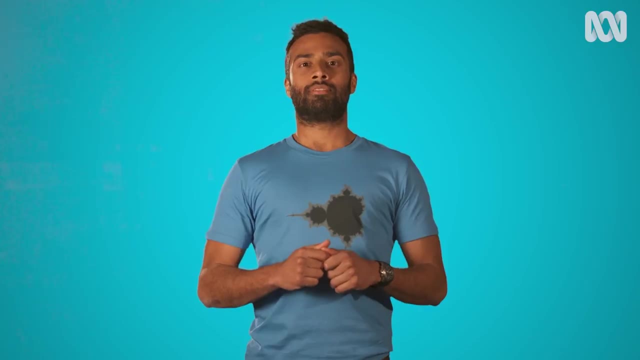 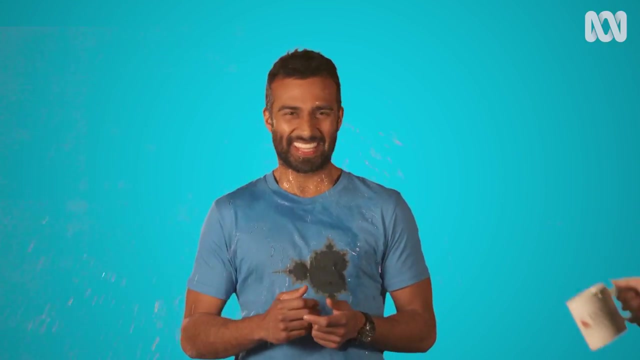 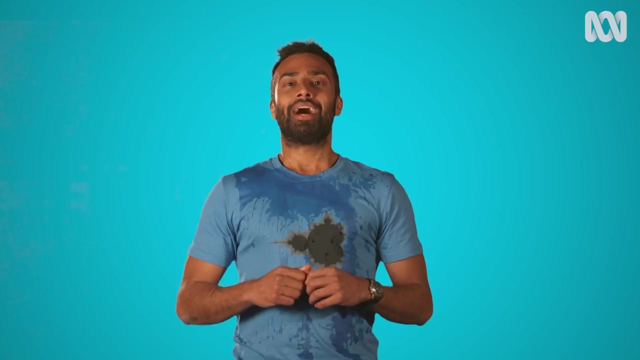 Hi, I'm Nige, and if I was a cloud, I'd be a cumulonimbus. How many times have you checked the weather and then walked outside to be greeted by this? Surely we're smart enough now to be able to predict the weather right. 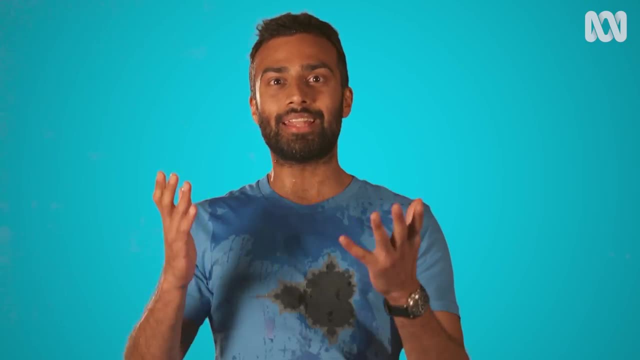 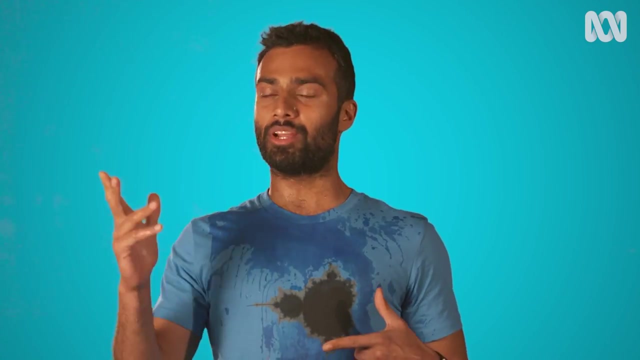 We can put people on the moon and predict complex movements of the solar system, but are still unable to say what the weather's going to be like next Tuesday. So why is it so hard to predict the weather perfectly? How does weather prediction even work? 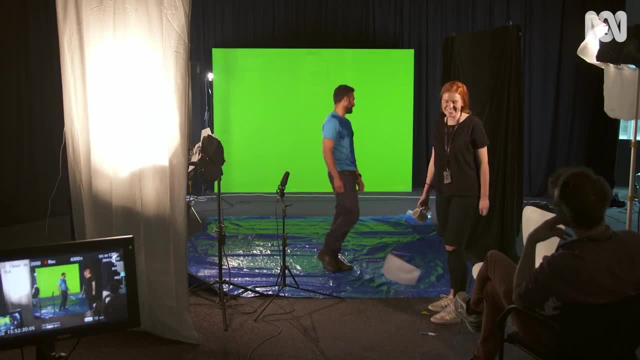 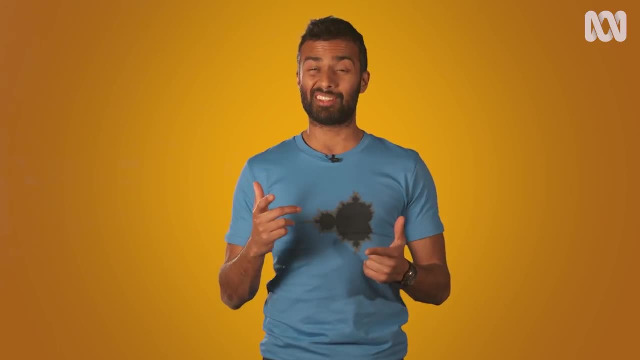 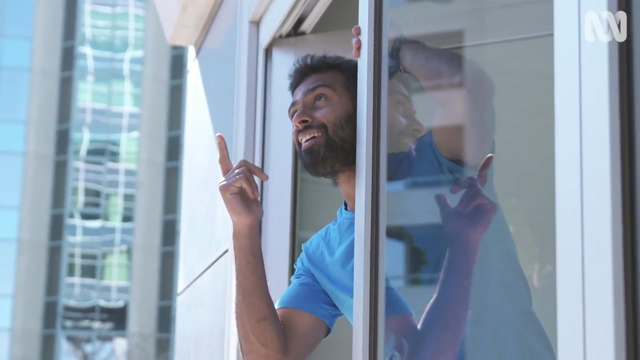 That last one is unnecessary. I'm out Right. so weather is actually amazingly complicated to predict. It's even harder than predicting the climate. What's the difference between weather and climate? Well, meteorologists say to stick your head out of the window for an hour, that's the weather. Stick it out there for a month. 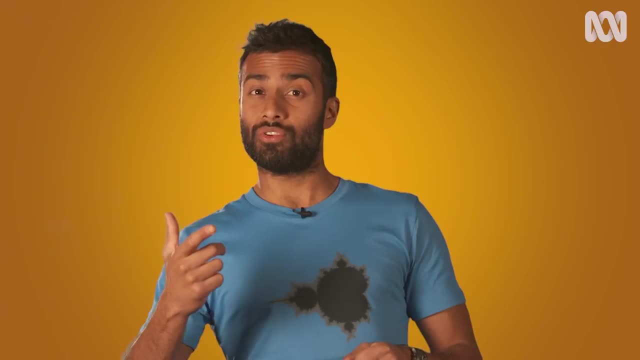 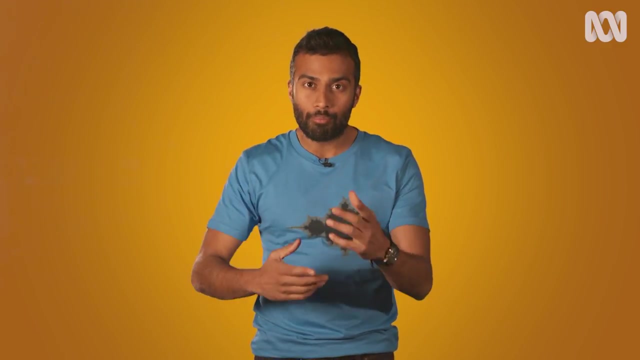 that's the climate. To predict the weather over the next few hours, through to the next few days, meteorologists don't just use one set of readings and give it a crack. They compile atmospheric conditions from around the world over a number of days, keeping an eye out for changes in pressure. 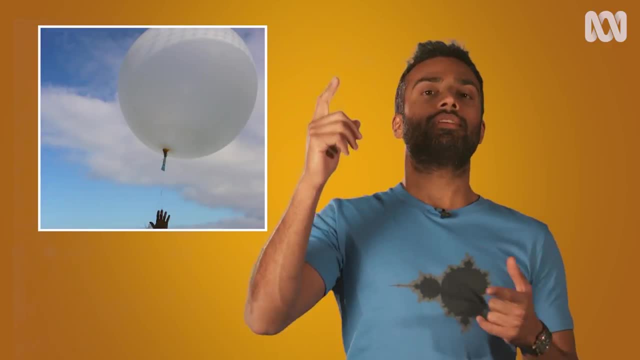 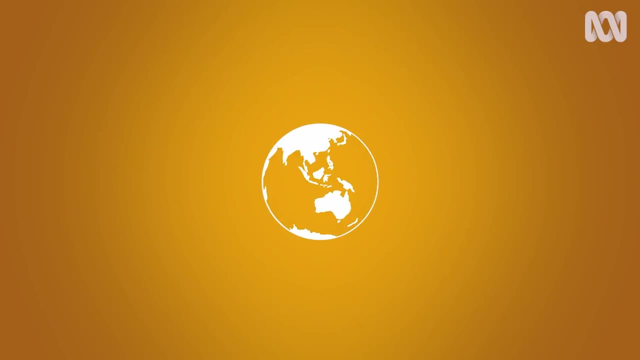 and temperature, and rainfall and wind speed. They send weather balloons into the sky and take weather readings from aircrafts and ships and monitor cloud patterns with satellite imagery. They're also assisted by historical readings and impressive numerical modelling that simulates how air, moisture and heat all flow over the Earth's surface. 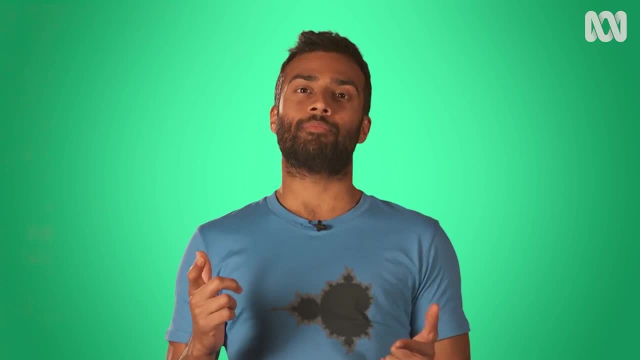 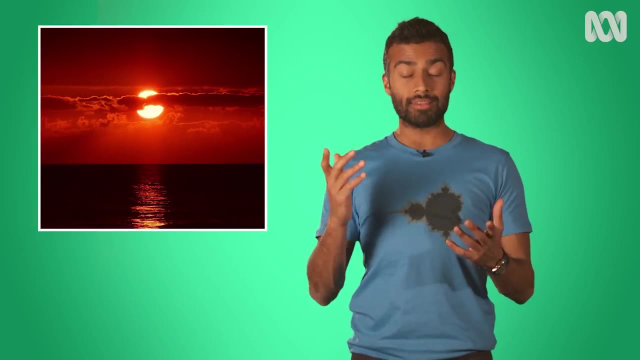 That's the weather. People have been predicting the weather for millennia and some of the sayings that have made it into folklore have solid basis in science. Red sky at night: sailors take delight. Red sky in the morning: sailors take warning. 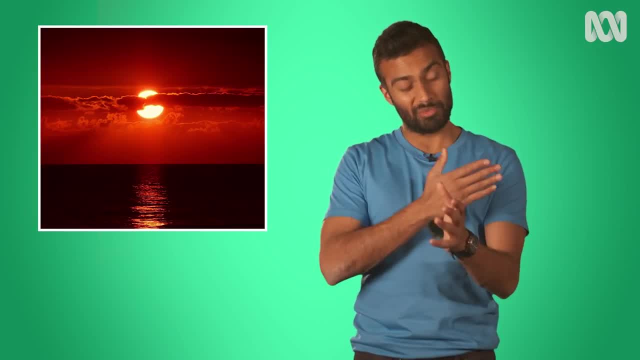 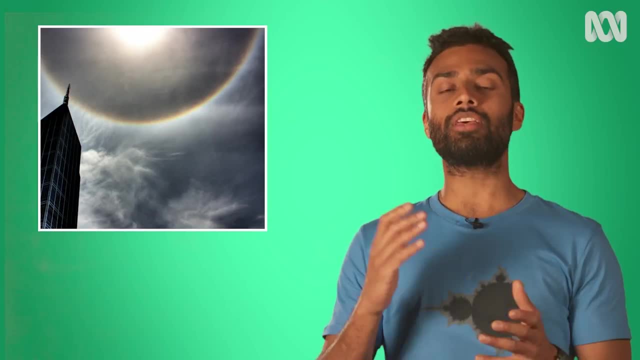 refers to the positions of clouds at sunrise and sunset and the fact that weather systems generally travel west to east at mid-latitudes. A ring around the sun or moon means that rain will come and soon tells of ice crystals in the upper atmosphere, which are often an indicator of an approaching low pressure front. 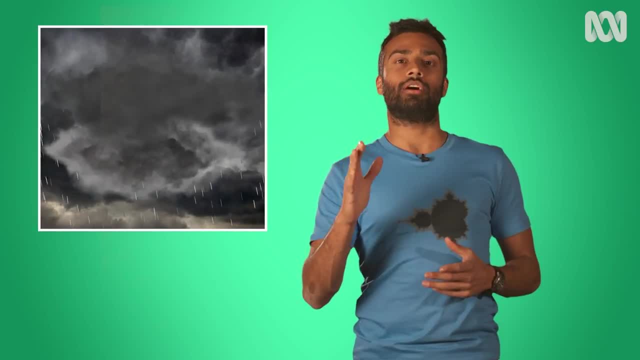 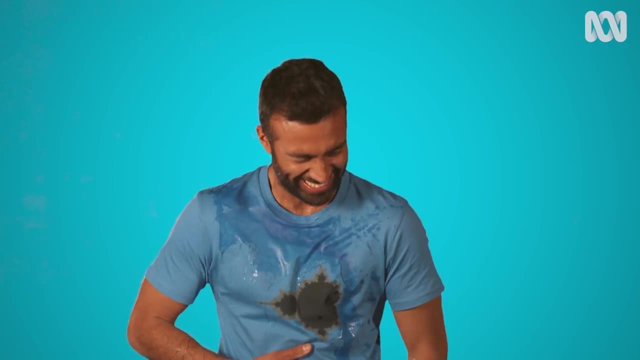 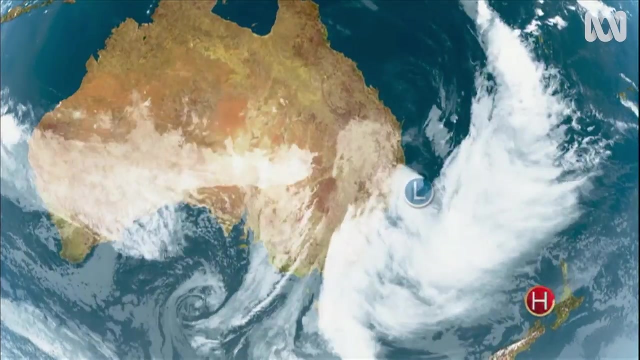 If the clouds move against the wind, rain will soon follow. references wind shear, which is instability between the upper and lower parts of the atmosphere and a good predictor of rain. But just how accurate are forecasts for letting us know if we should be packing some sunscreen? 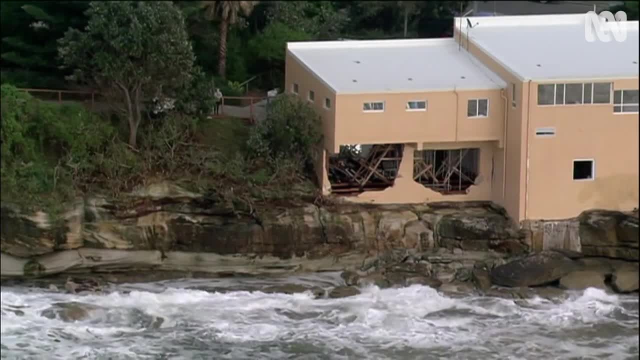 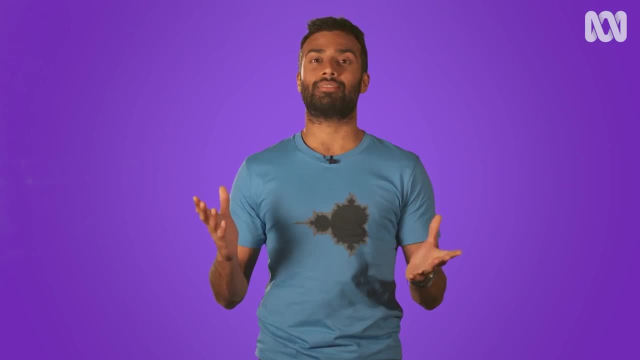 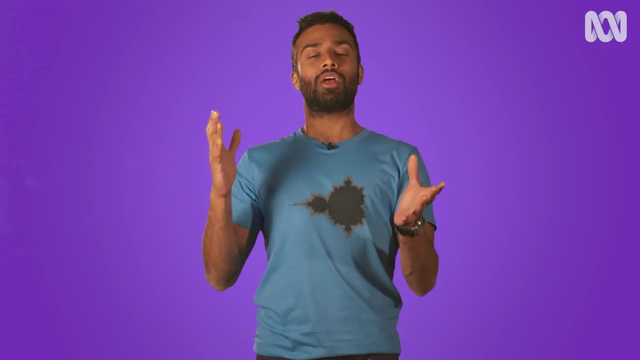 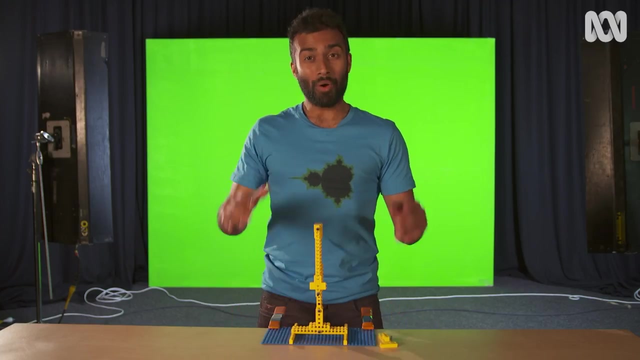 And it's certainly true. I read a kid's book about it. It's because of a branch of physics and maths called chaos theory, which looks at complex systems and how they are very sensitive to initial conditions. A way of demonstrating chaos theory is with a pendulum. If I let this single pendulum 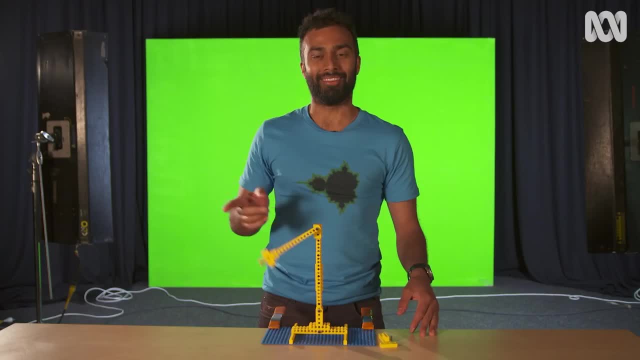 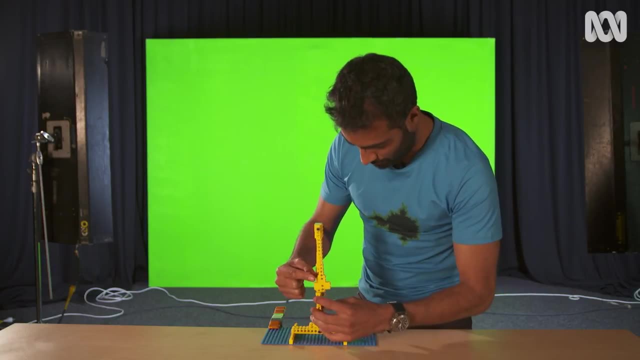 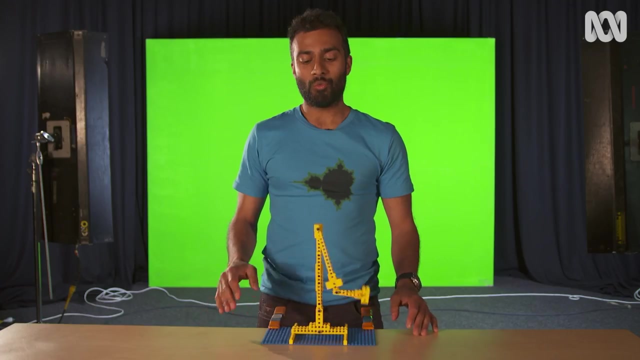 drop, its behaviour is very predictable. But if I increase the complexity of the system by adding a second arm to make a double pendulum, its behaviour suddenly becomes very difficult to predict, With tiny changes in initial conditions how I pushed the pendulum at the start leading 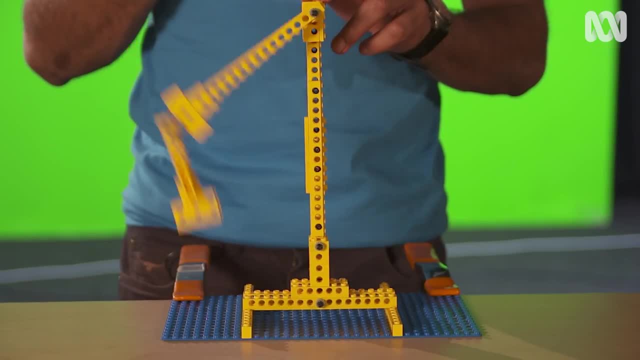 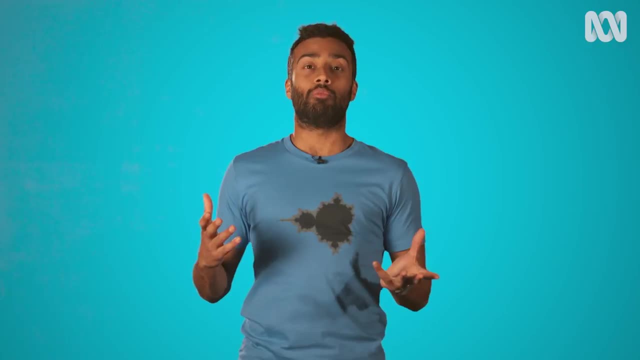 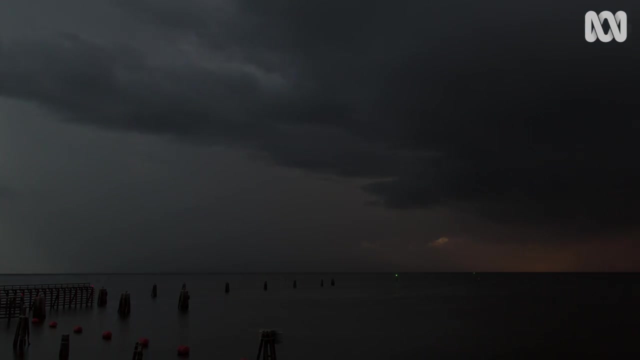 to very different outcomes at a later time. Scientists have found this sensitivity to initial conditions and resulting chaotic behaviour in many aspects of our lives, from prices on the stock market to fluctuating animal populations, to fractal shapes like the one on my shirt and, of course, with something as complex as the weather. So with that in. 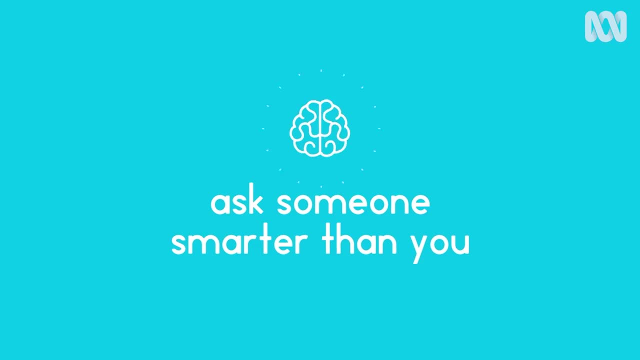 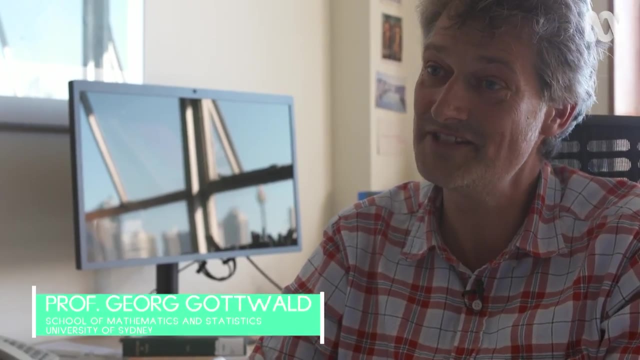 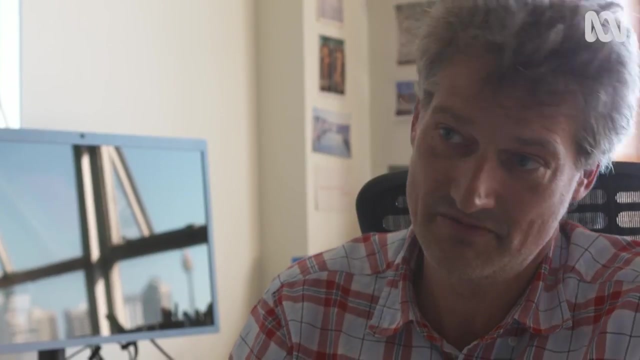 mind. how accurately can we expect to predict the weather? Are we getting better at understanding complex systems like the weather? Well, yes, there's two aspects. First of all, we can do better forecasts, but that's mainly due to faster computers and also more observational data, which is probably the main reason why. 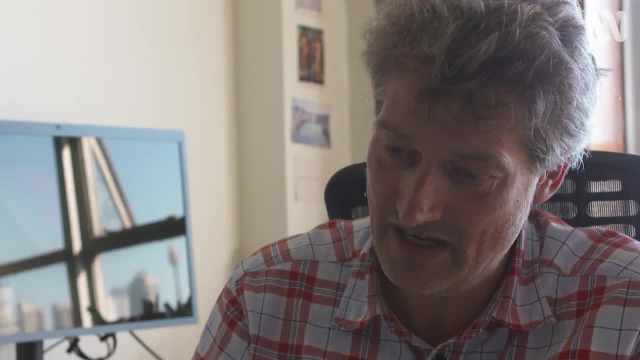 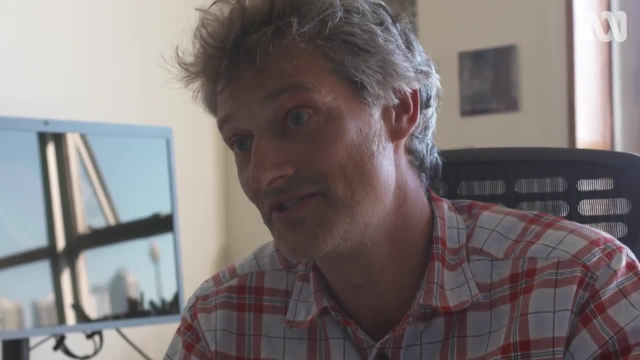 we have a better forecast now, But we also have to develop better methods to deal with not having enough data and integrating the equations that will give us the forecast. So if you want to see a better forecast, you can use a big-sized scale If you want to. see a better forecast, you can use a big-sized scale. So if you want to see a better forecast, you can use a big-sized scale. So if you want to see a better forecast, you can use a big-sized scale. So if you want to see a better forecast, you can use a big-sized scale. 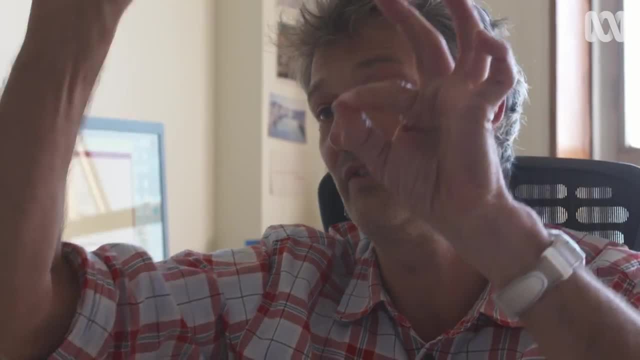 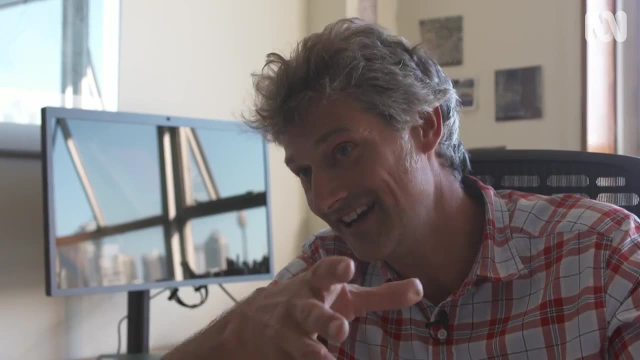 If you won't solve the system, then you have to discretise your space. You can't solve the temperature everywhere. you have to decide at certain discrete points, only at certain discrete times. So examples are high and low pressure fields. I mean now we can actually do pretty good prediction. We can now do three days pretty well. Then El Niño is another large scale structure we can treat in some sense on certain timescales, predicatable Of course. on much longer timescales also, the instability of those systems depends.